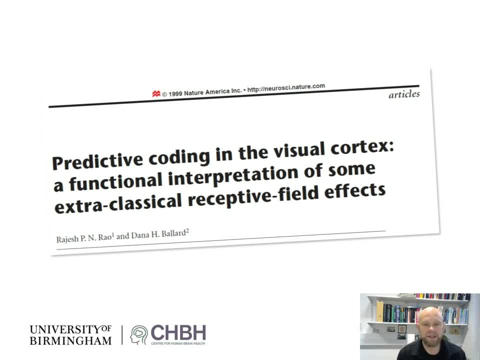 also generalize to language comprehension, And the basic idea is also that our brains constantly are making predictions, attentions and predictions. Thank you. It can be compared to the sensory input. One purpose of these predictions during language comprehension could, for instance, be to speed up processing, sort of to give the comprehension. 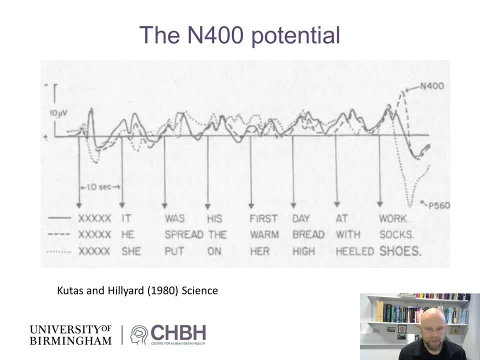 of language, a head start. So indeed there have been a lot of discussions on predictions also investigated by electrophysiological approaches. So you might all be familiar with the N400 potential. So this was a first finding done by Kudes and Hilyard back in 1980.. For instance, if you are presented with the sentence he: 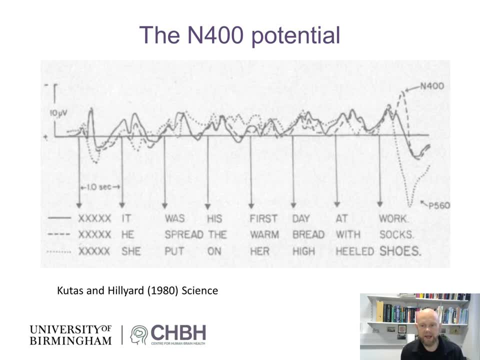 spread the warm bread with socks, Well then there is a violation to the expectations. when you hear socks right, This violation to the expectations leads to a strong N400 potential. that you see as a negativity, But, as we know, it is not always an argument. The conjecture: 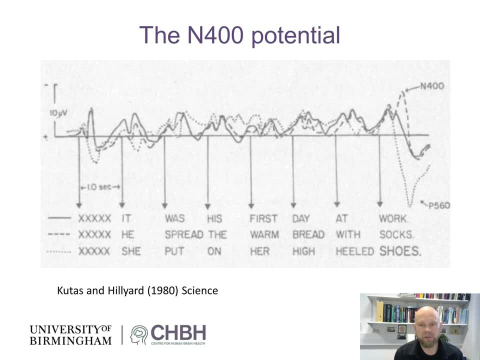 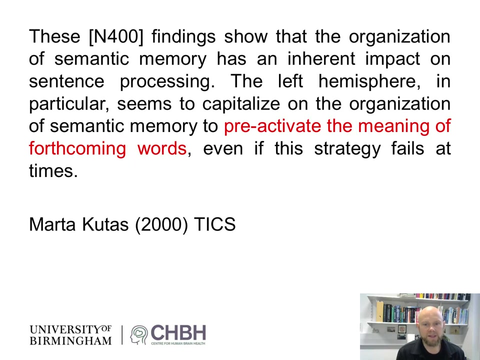 in the ERP about 400 ms after the presentation of the word. So what does this N400 potential mean or indicate? So, indeed, it has been proposed that the N400 reflects a violation to pre-activations of words during language comprehension. Now there's a debate to whether the N400 actually does reflect violations to predictions. 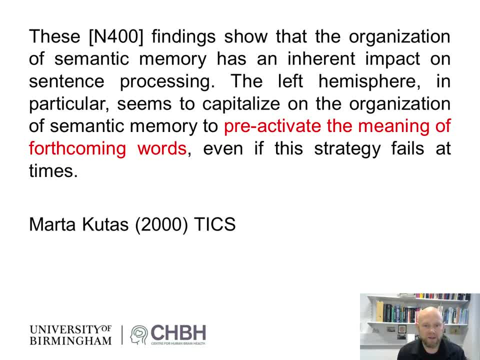 There's also the alternative explanation that the N400 reflects on some sort of updating process occurring after the word being presented, violating the context Now, unless there's a debate going on. but what we would like to argue here is that if you want to study pre-activation or prediction, 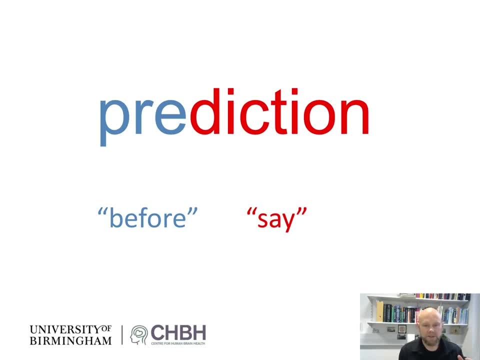 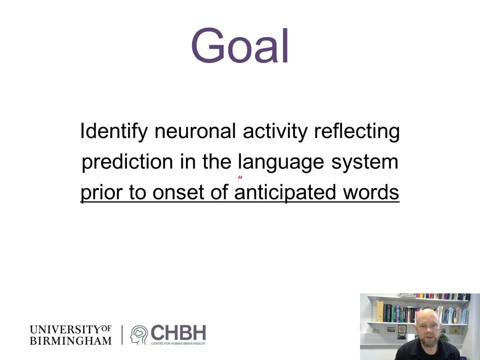 Well, Basically, you have to look at the brain activity before the critical word, not after, as one does with the N400.. And I'm going to tell you how we have been doing this with MEG recordings. So, basically, the goal of this study is to identify the neuronal activity reflecting 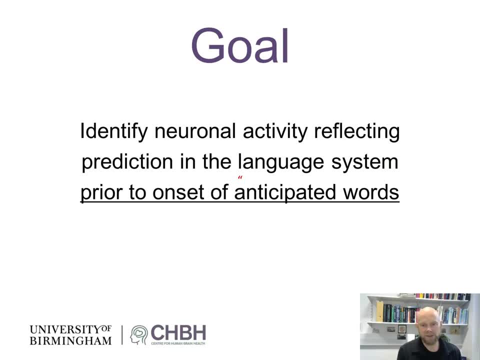 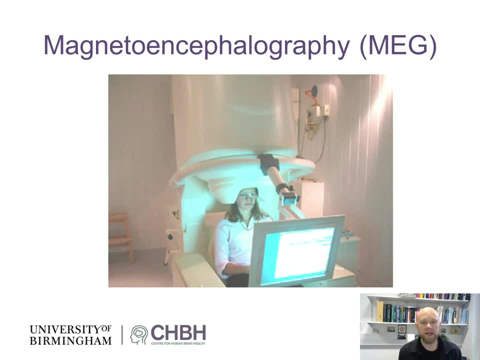 the predictions in our language system prior to the onset of the anticipated words, And to investigate this we use MEG. So MEG has this ability that allows us to record the brain activity on a millisecond time resolution, but it also allows us to localize where in the brain the activity of interest. 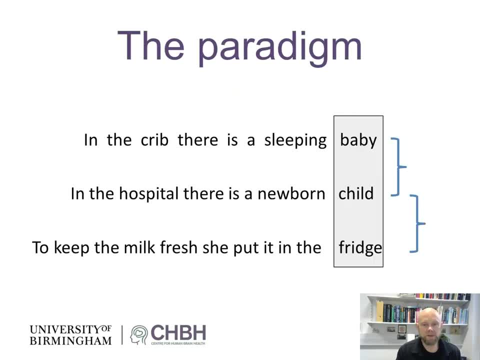 is being generated. So what we did was to design a study in which the last word could be predicted. So what you see here is that in the crypt there is a sleeping baby. In the hospital there is a newborn child or baby. That's the second sentence. 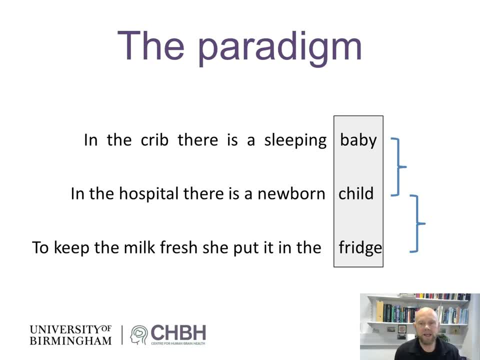 And in the crypt there is a baby. So these two sentences are predicting the same last word. The third sentence here is: to keep the milk fresh, she put it in the fridge. So the second and the third sentence are predicting different words. So basically, what we have been looking at is the brain activity just prior to the onset. 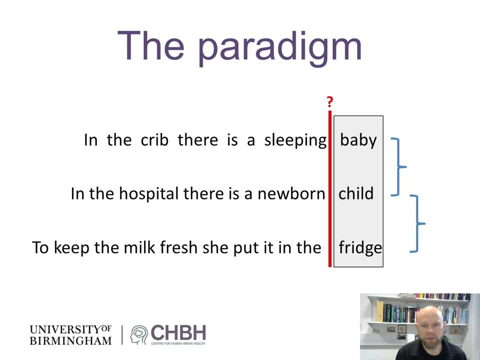 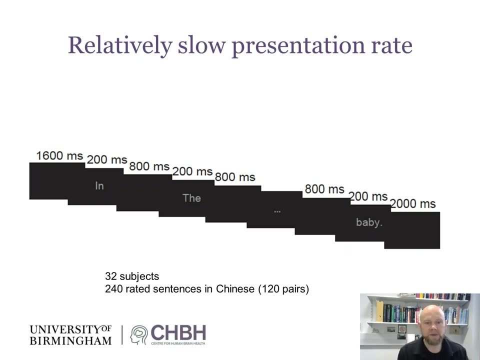 of the last critical words in the sentence, And the core prediction was that this brain activity should be more similar when similar words are being predicted as compared to when different words are being predicted. So what we did, or what Linh did, was to present sentences, in this case in Chinese, because 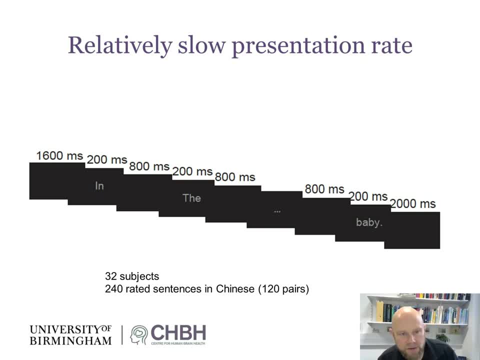 the study was done in China, So it was written words. They were each presented for 200 milliseconds and the rate was one word per second And it was always the last word that was being predicted. So very simple paradigm here. And of course, we had pairs of words where there were 120 pairs that predicted the same. 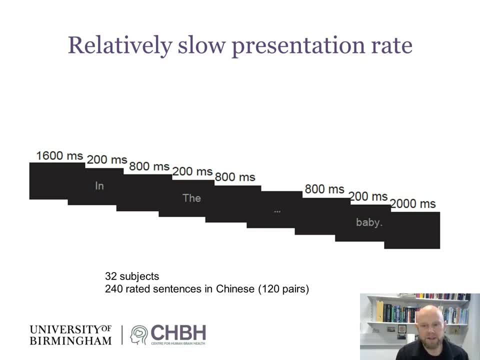 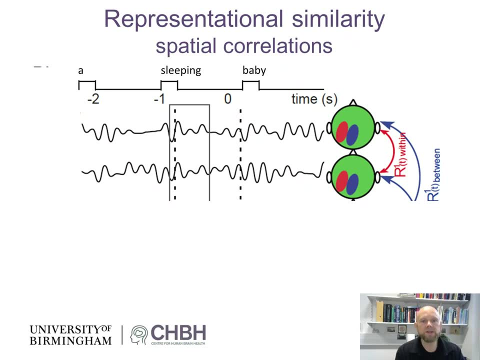 last word That allows us to compare sentences where the same word versus different words were being presented, And this is exactly what we see here. So the logic of the analysis is that we look at the brain activity recorded with MEG as the words are being presented. 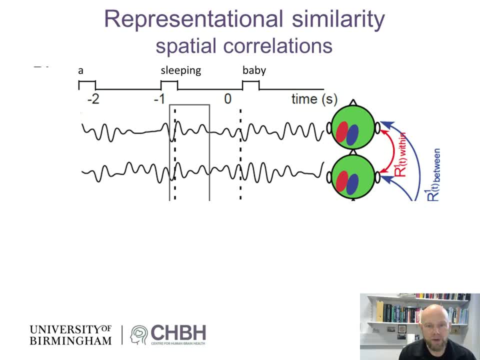 Then we look at the brain activity just before the predicted words, And then we look at the spatial distribution, the topography of the brain activity, And what we argue is that if the same word is being predicted, then the topography should look similar as compared to when two different words are being predicted. right, 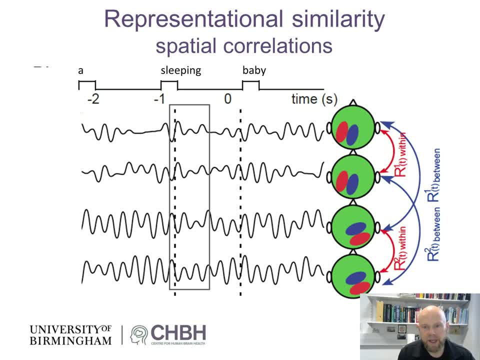 So the two first sentences could be predictions for baby, baby. The two last sentences could be for fridge, fridge. So for these pairs the brain activity should be similar. But they are not the same. So we look at the two first sentences. 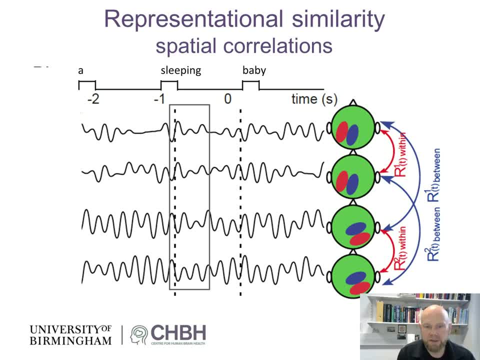 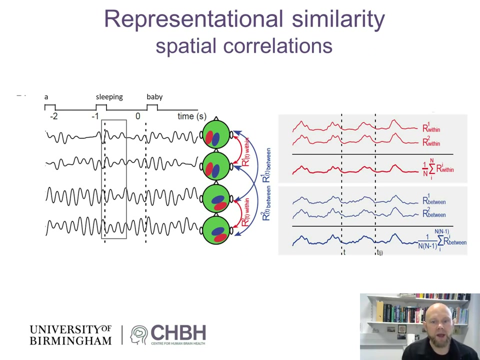 but with respect to baby versus fridge, these predictions, the topographies, should be relatively different. So, basically, we looked at this similarity by simply calculating the correlation over sensors in the brain activity, And this then allowed us to look at the difference in correlations between within predictions. 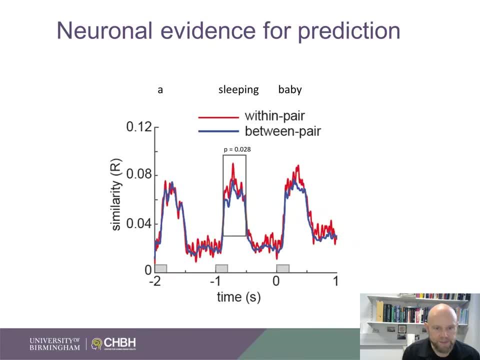 versus between differently predicted words, And this is what the data looked like. As you can see, the brain activity or the correlations here are going up and down with the presentation of each word. So the bulk of this going up and down is due to the evoked responses generating brain activity. 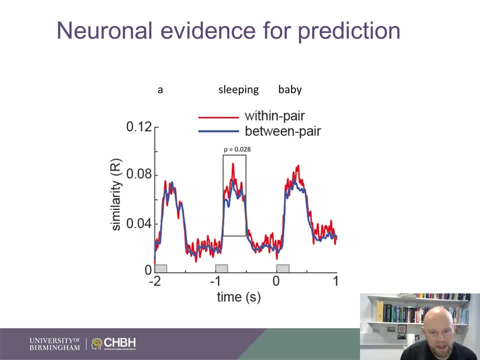 resulting in high correlations. But the key finding here is that we now can compare the within pair to the between pair with respect to upcoming words right And when the same words- the within pair- is being predicted. lo and behold, we see the correlations being stronger. 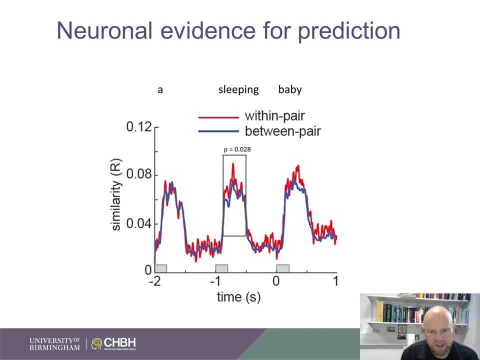 as compared to when different words are being predicted. That's the blue line right. So it's a difference in correlations here being important, And what you should also appreciate is that we now can compare the within pair to the between pair with respect to upcoming words. 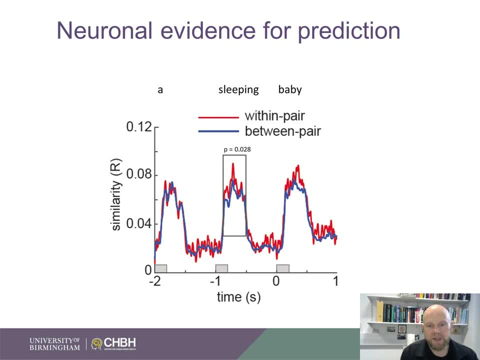 And what you should also appreciate is the time course here. So at time zero is when the predicted word is coming on, And at time minus one, that's when the word just prior to the predicted word is being presented. And what you should note here is that these differences in predictions 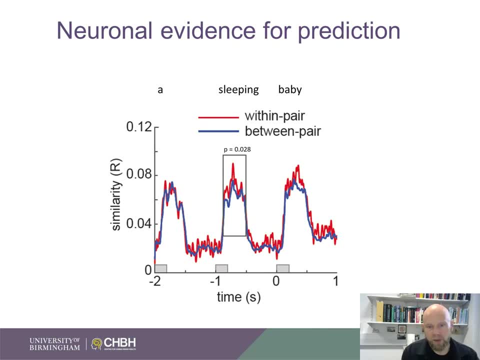 are occurring quite early, meaning as early as possible, when you can predict last word. In fact, we did actually initially anticipated that these predictions would be strongest just prior to the onset of the last word. So this is the difference here: prior to the onset of the last word. 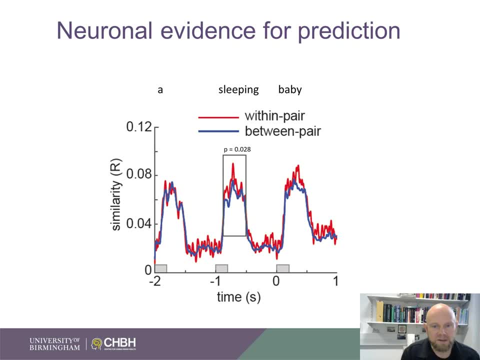 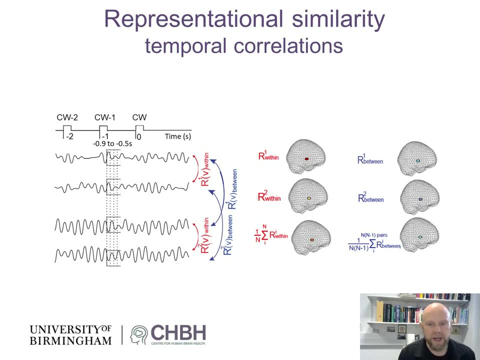 This is not the case. It seems the brain is making these predictions as early as possible. Now it turns out that we can also try to localize where in the brain these predictions are occurring, And we have been doing this, looking at temporal correlations rather than spatial correlations. 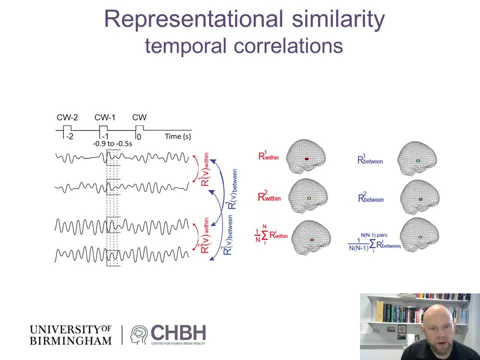 And what you should note here is examples of ongoing brain activity. So this could be from sensors, but it could also be from spatial filters, from the full brain volume, right. So what we have been doing is to use a beamforming approach to isolate the activity. 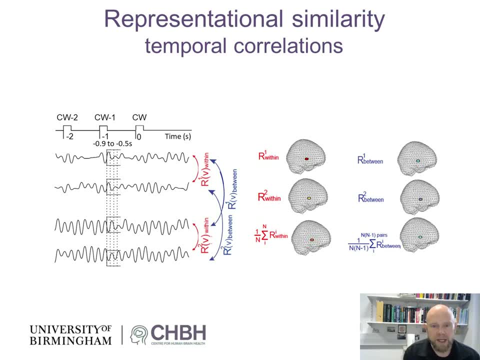 from each source or grid point, if you will, in the full brain volume, And what we then can do is to look at the time courses and then look at the correlation over time courses. So before we looked at the correlation over sensors, now we look at the correlations over time. 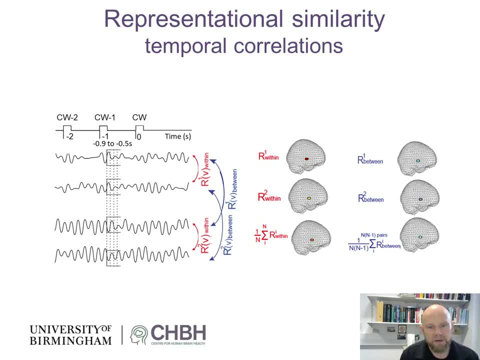 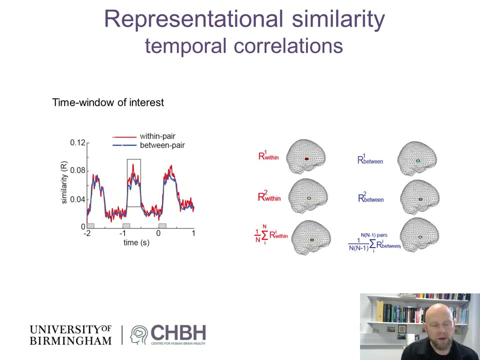 And then we can do the same trick of comparing within versus between correlations And then we can ask: where is the difference largest between? when comparing within versus between? And we do that for the time window where we found the predictions being strongest before. When we do that, we find these predictions. 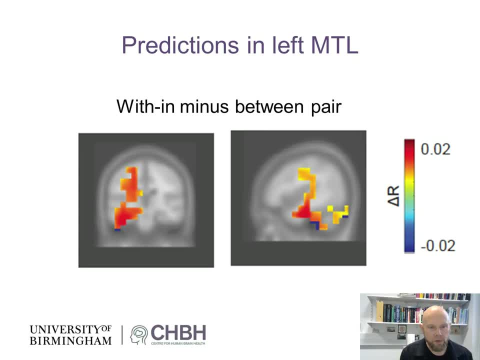 to be strongest in the left hemisphere. Furthermore, we find the predictions to occur in the medial temporal lobe in a bit, And also these predictions are including the hippocampus. So this is something we are quite excited about because typically in language research, 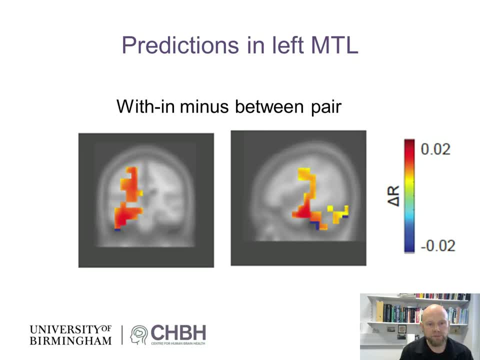 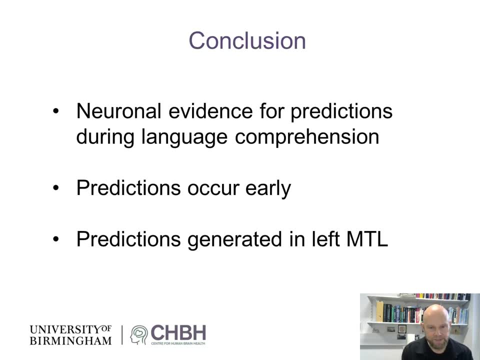 the hippocampus is not really considered. Now we find support for the notion that the hippocampus might be involved in doing predictions during language comprehension. So I'm going to finish here by concluding. We have found the evidence- normal evidence- for predictions of preactivations during language comprehension.